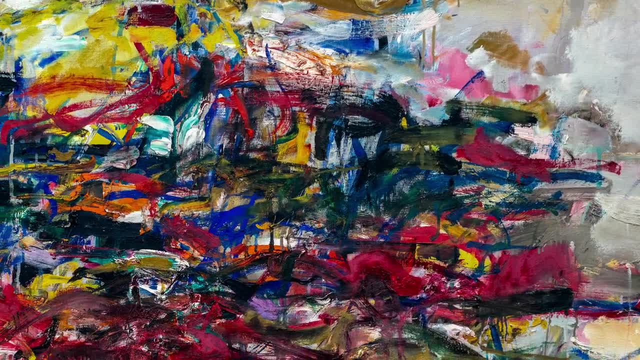 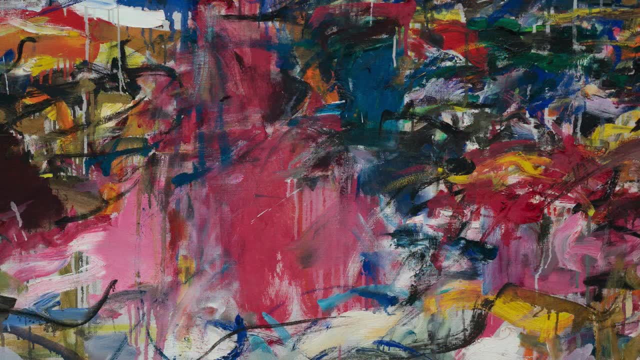 The denser central passages feel activated to me. The word I would use is energy. There seems to be a colliding of color and stroke and tone. I'm really drawn to the pink, which is largely underneath those blues that you noticed. There's a section of the pink. 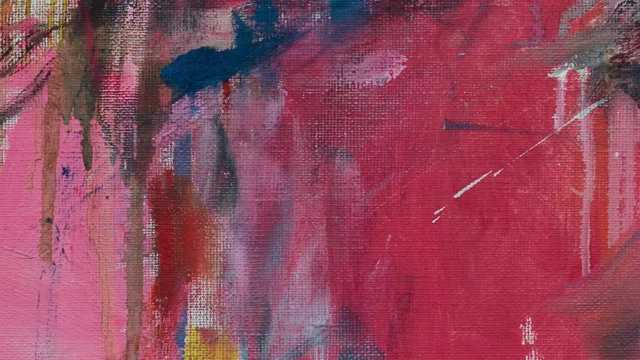 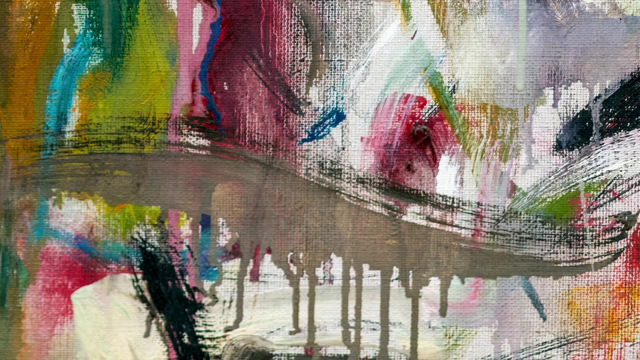 that almost seems to reveal the linen, and then I start to look for that same feature elsewhere and I see it in other spots as well, with aqua or blue or yellow, And some areas seem very intentional where we can feel the movement of the artist's hand. 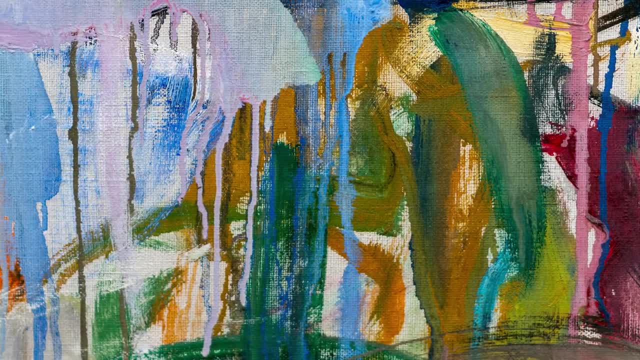 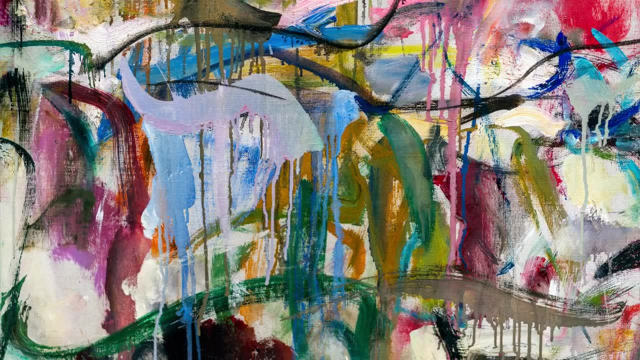 and then other areas feel rather accidental where the paint is dripping down, And so, all of a sudden, this painting feels archeological, as if we're able to reveal earlier moments in its creative process. Let's think about this title: City Landscape. 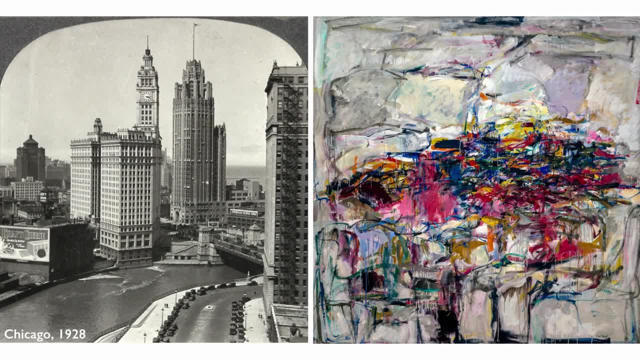 When you look at the painting do you start to conjure up a memory of a city landscape? The title is tricky for me because it closes down the openness of the meaning of the painting. It's a little bit like when you read a book. 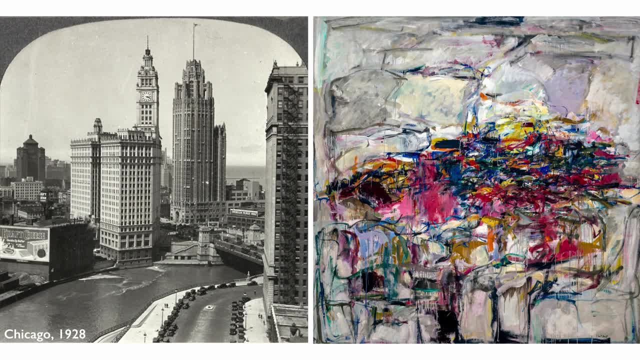 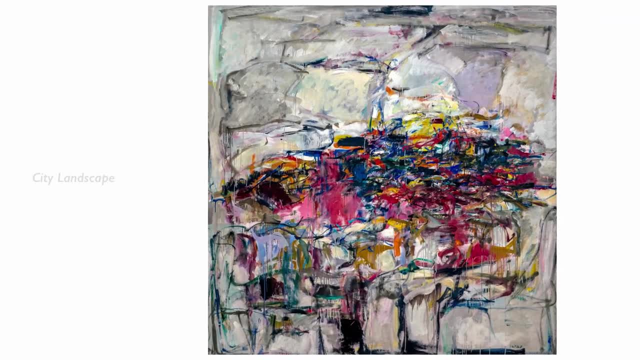 You have your own ideas about what a character looks like, but then you go see the movie and a director has made that decision for you In an interesting way. you lose something. But I wanna challenge the idea that it can't also invite us in. 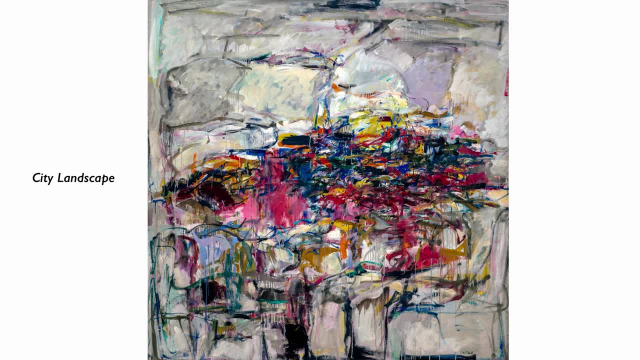 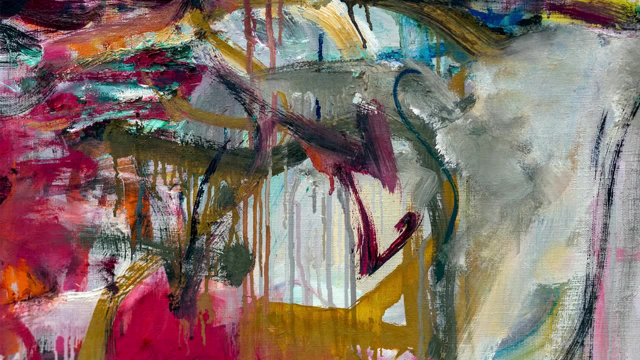 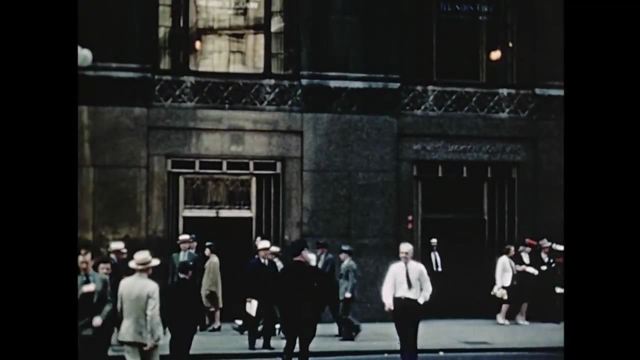 to bring our own personal interpretations and let just the prompt of city landscape open up a new avenue for exploration of this painting. There's such a variety in the application of paint. All of those differences make me think about the bombardment of all the different kinds of things that one. 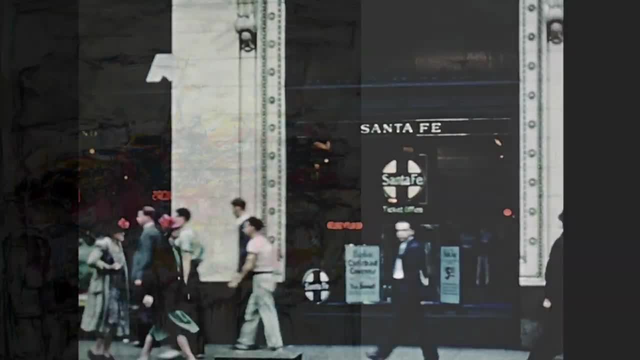 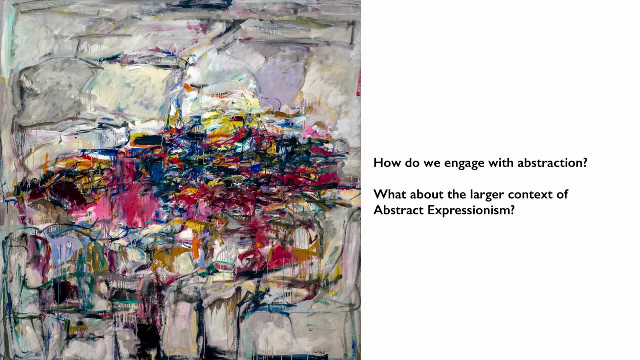 experiences in a city. It's a kind of cacophony. There are different questions that this painting poses for us. One of them is: how do we engage with abstraction? How do we understand it in the larger context of abstract expressionism? Joan Mitchell, although she comes from Chicago. 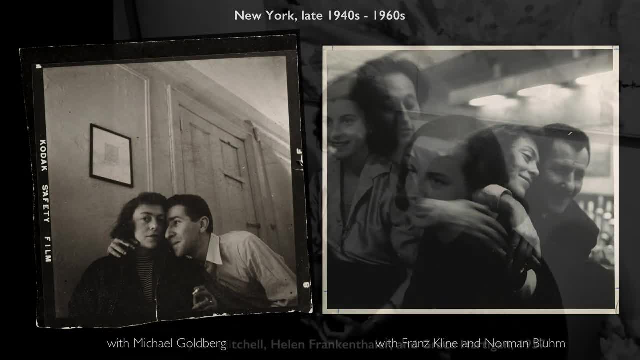 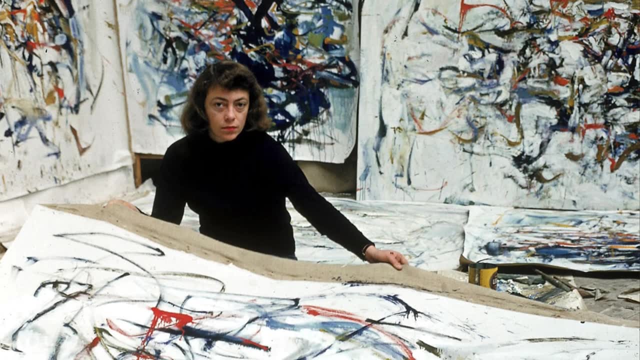 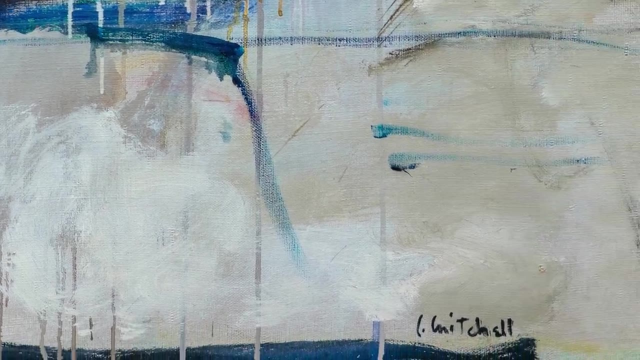 goes to New York, eventually to Paris, and has lived through the Second World War and is spending time with abstract expressionists. she is throwing off the yoke of representation that had ruled painting for centuries, and there was a tremendous assertion of freedom of exploration.